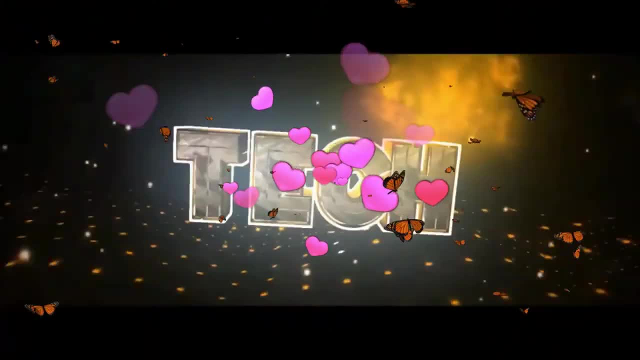 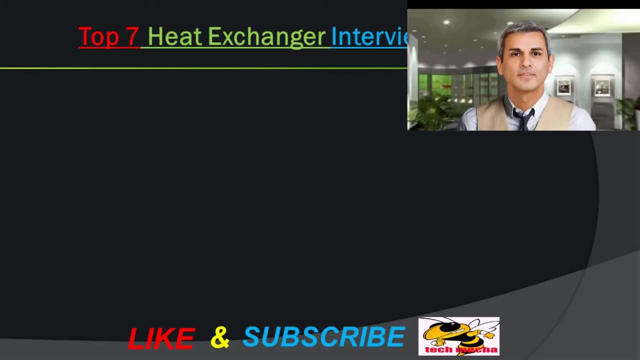 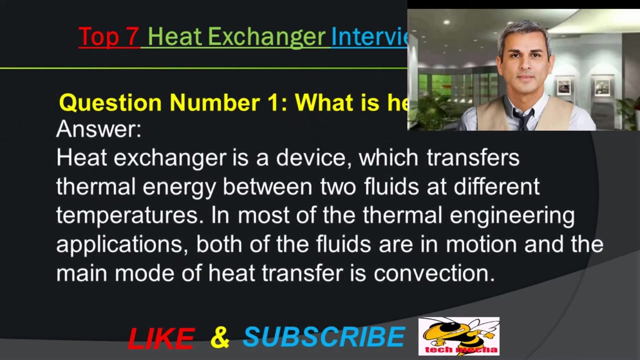 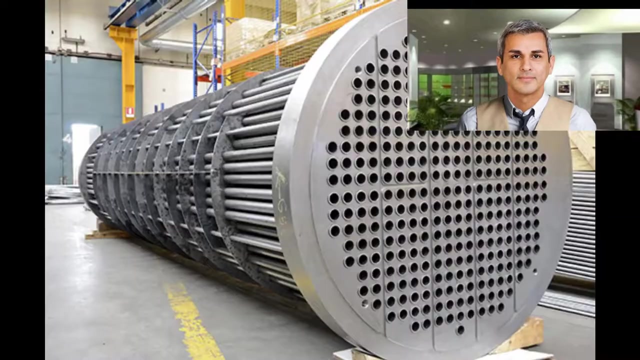 Question number 1,. what is heat exchanger? Answer: Heat exchanger is a device which transfers thermal energy between two fluids at different temperatures. In most of the thermal engineering applications, both of the fluids are in motion and the main mode of heat transfer is on. 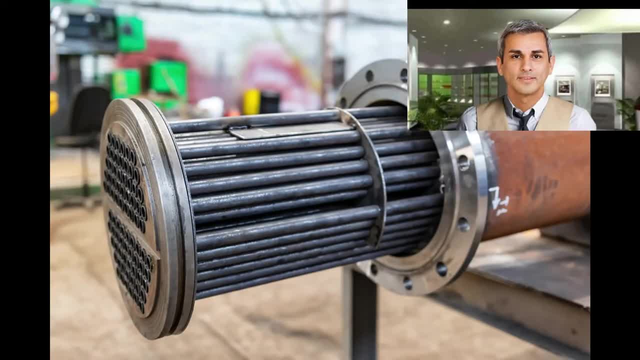 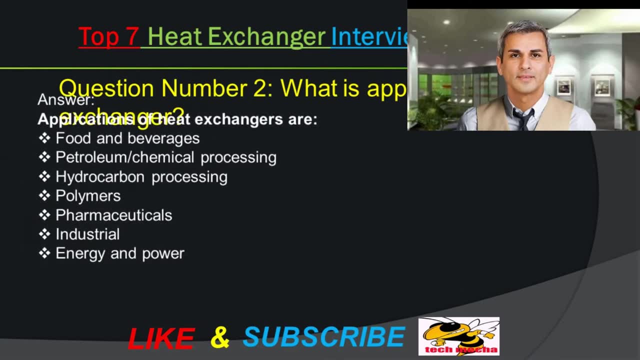 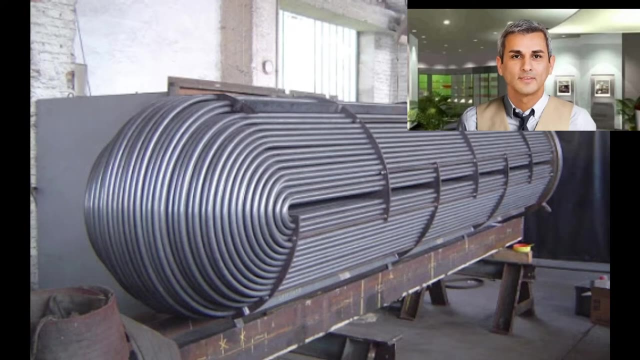 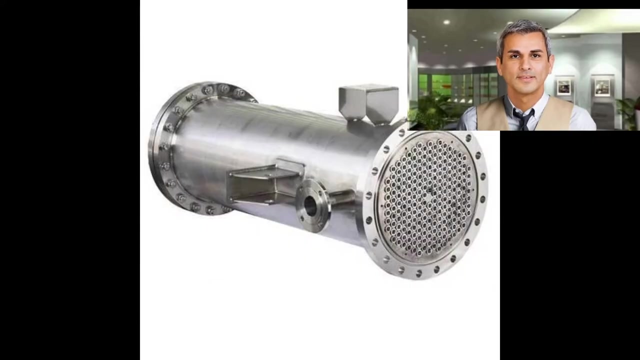 Transfer is convection. Question number 2, what is application of heat exchanger? Answer: Applications of heat exchangers are Food and beverages, Petroleum slash, chemical processing, Hydrocarbon processing, Polymers, Pharmaceuticals, Industrial Energy and power. Question number 3, what is heat exchanger? Answer: Heat exchanger is a device. 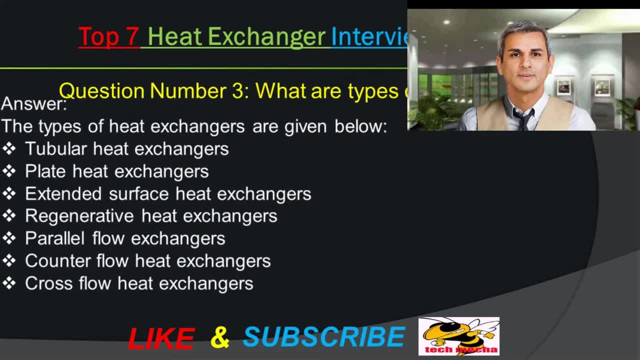 which transfers thermal energy between two fluids at different temperatures. In most of the video tutorial we share common top 7 heat exchanger interview. This top 7 heat exchanger interview question is best question for interview. What are types of heat exchanger? Answer The 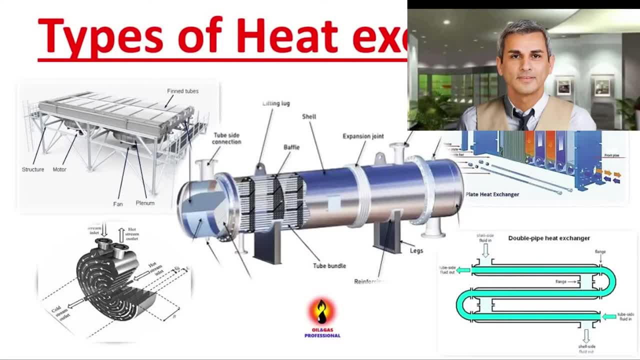 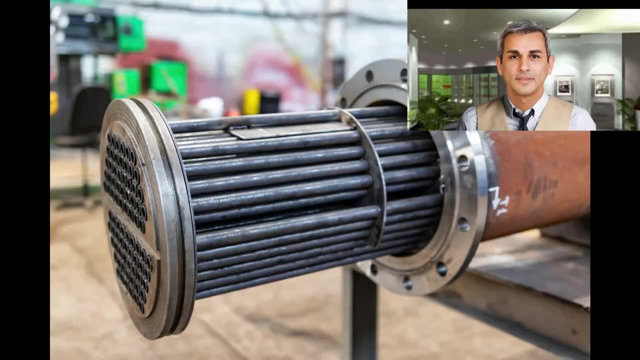 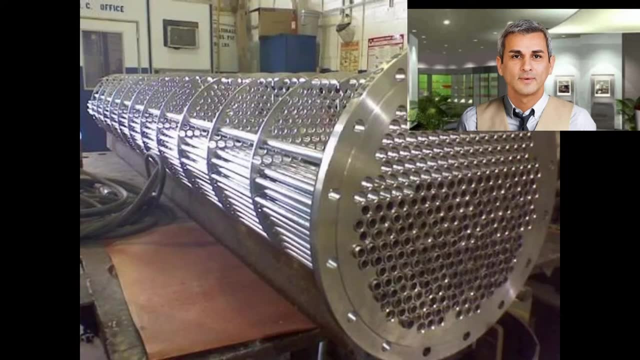 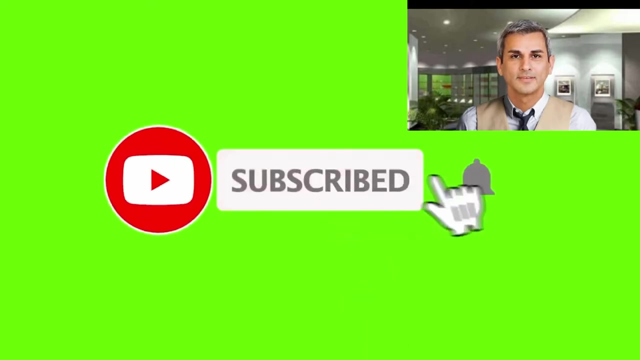 types of heat exchangers are given below: Tubular heat exchangers. Plate heat exchangers. Extended surface heat exchangers. Regenerative heat exchanges. Parallel flow exchanges. Counter flow heat exchanges. Cross flow heat exchanges. click the bell icon for update notification. Also like comments and subscribe my video channel. 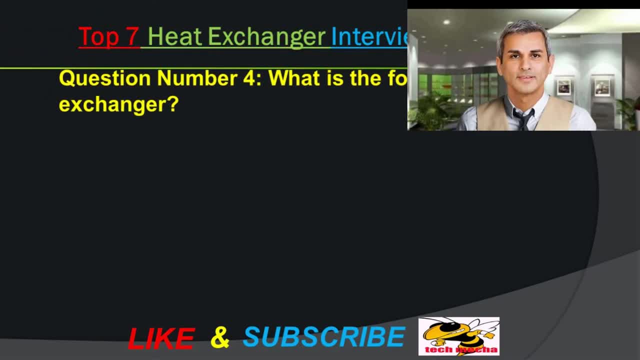 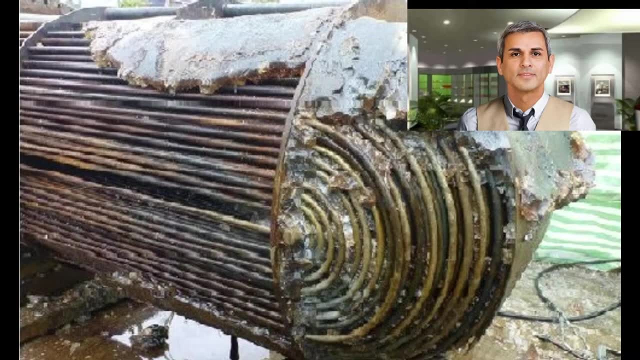 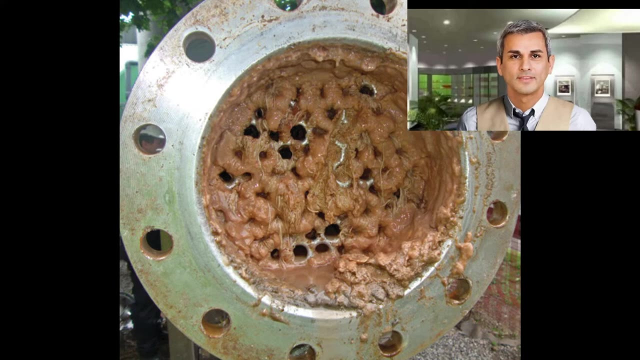 Question number 4, what is the fouling factor in a heat exchanger? Answer: Fouling is a general term that includes any kind of deposits of extraneous material that appears on the heat transfer surface during the lifetime of the heat exchanger. Fouling reduce heat transfer across the 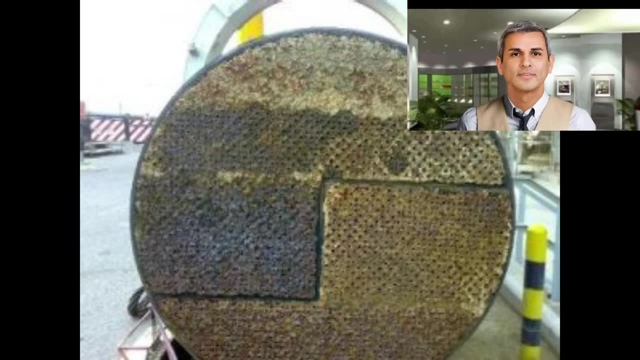 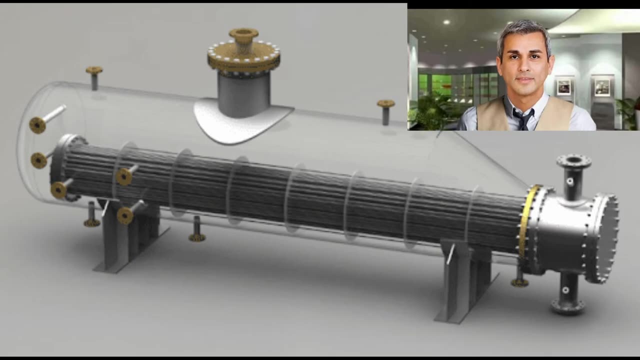 exchanger surface, hence reduces efficiency of the heat exchanger. The fouling deposits also reduce flow cross-section area, causing a pressure deferential across the heat exchanger which, in turn, increasing on the fan power required It, might also eventually block the heat exchanger. 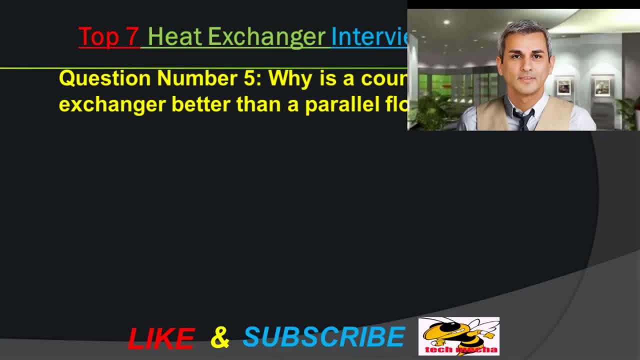 Question number 5, why is a counter flow heat exchanger better than a parallel flow heat exchanger? Answer: In counter flow arrangement, the heat exchanger is more efficient than the parallel flow heat exchanger. Answer: In counter flow arrangement the heat exchanger is more efficient than the parallel flow heat exchanger.